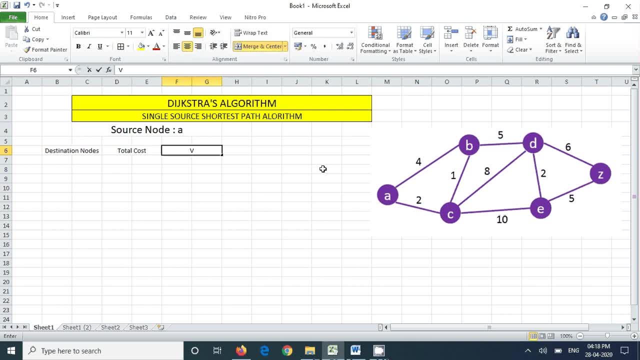 And there is a via node, From which node you are coming, The one previous to that via. So we will be having the nodes B, C, D, E, Z. So we have a total of 5 nodes which are destination nodes. Source node is A. Source node is A. 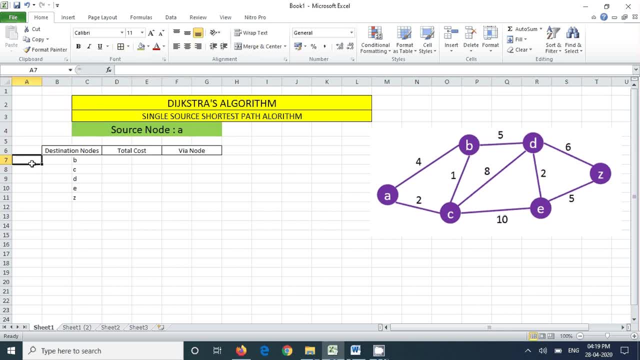 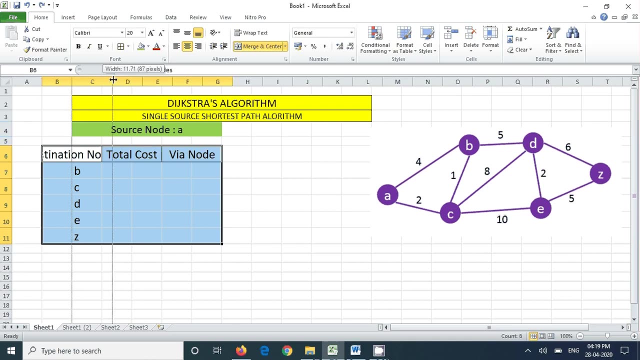 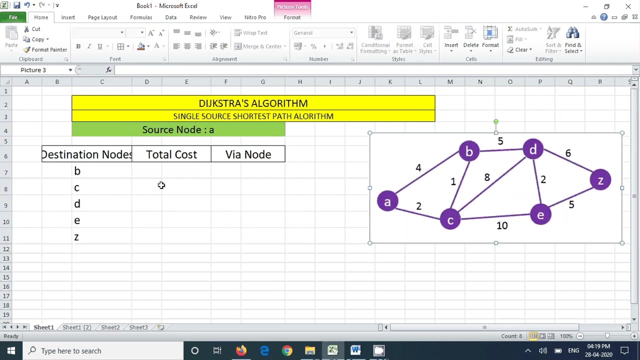 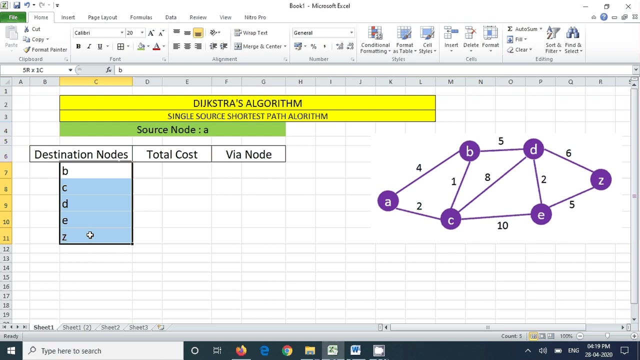 We are having 5 destination nodes: B, C, D, E and Z. So we are going to work for this, How the path is found out. So we will be having B C, D E Z. We have a total cost of B C, D, E, Z. 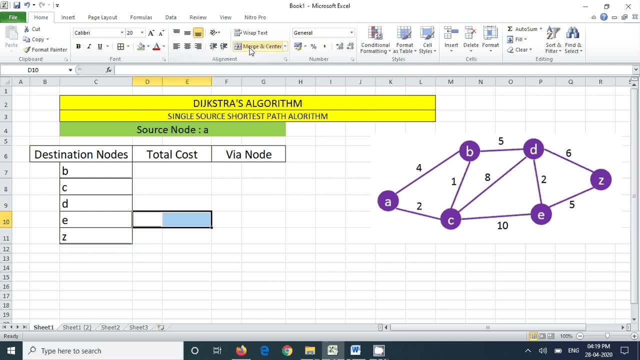 So we are going to work for this, How the path is found out. B C D E Z. So we have a total cost to come to that node. B C D E Z. Total cost to come to that node. 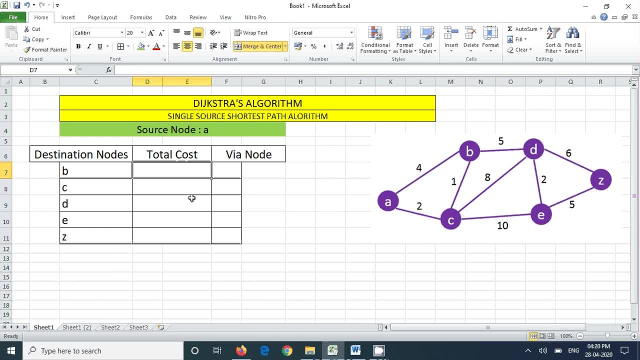 B, C, D E Z. B, C, D E Z. Total cost to come to that node a. that's why so initially it's all infinity, so we'll just put infinity for all these nodes. it's all infinity. so from a to reach b, c, d e, z, it's all infinity. so y a node is also. 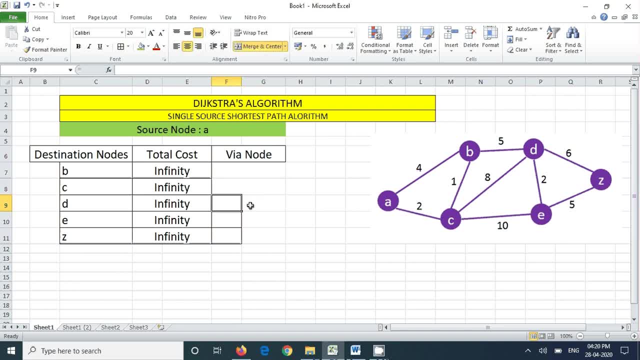 as of now, it is empty. so first initial startup is you have to put infinity for every node, every destination node, from a, from a to every destination node. it's the infinity cost, total cost. this is total cost. so we will start with the scanning from a. we are standing in a we. 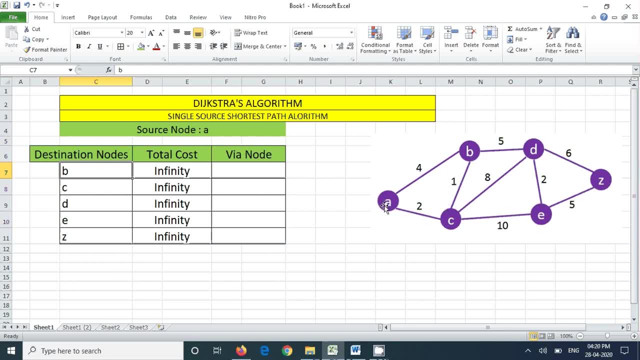 have to find the shortest path to all the other nodes from a. we are standing in a, so we scan. we scan means we just find out where the a is connected directly. so that's what we scan from a. so which is so? whichever is we are discovering, we will be updating a table. 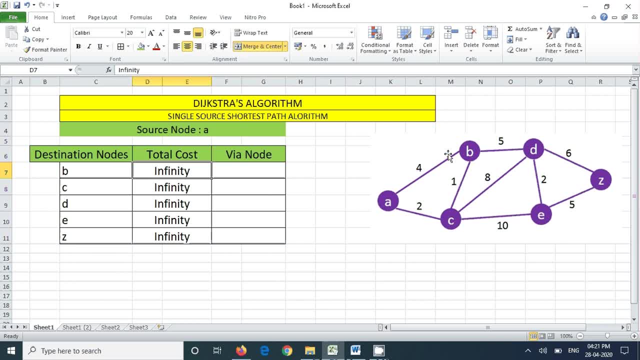 with So b. from here I can go to B with the cost of 4. so 4 is less than infinity value, then only I will replace: is that infinity? so if it is something less, then we will replace the bigger one. so 4 is less than infinity, so we replace infinity with 4. 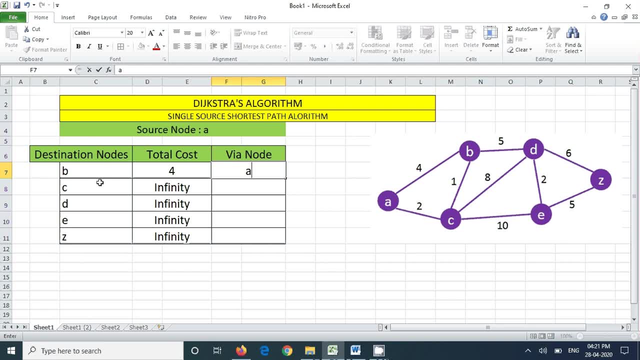 then the via node is a. so to reach B the cost is for the previous node. the previous node is A, the previous node to B is A. then the B A can go to C also directly with the cost of 2. 2 is also less than infinity, so I will put 2. 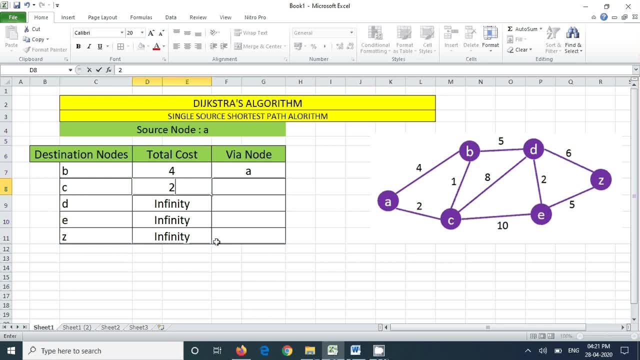 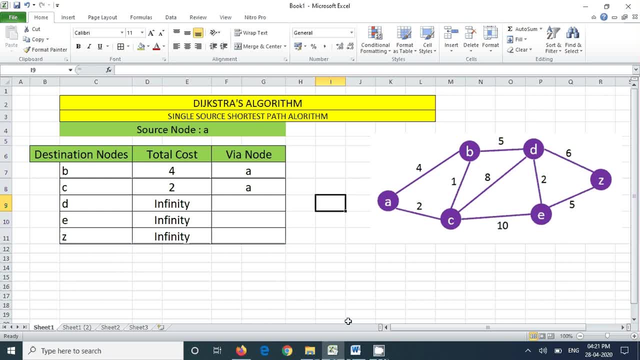 can from what, which one we have to add to the answer. so out of these node, the Dijkstra's algorithm says you have to follow a greedy procedure. greedy procedure is: whichever is smaller, whichever the total cost is small, smaller, then you have to select that one. so it's the smallest in the discovery. so 4: 2. 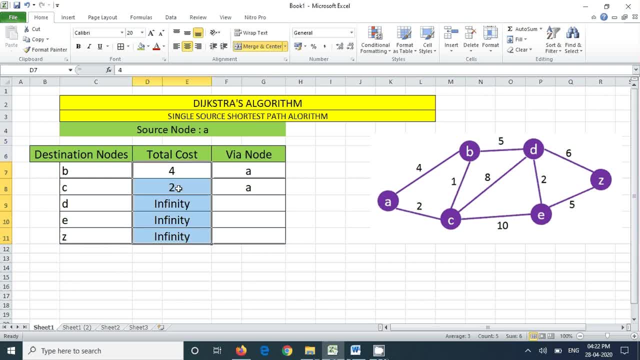 infinity, infinity, infinity. so out of these five values, 2 is the smallest. this you have to take it and fix it as an answer, because we are building part by part. so this is a good solution. so this is a good solution. so this is a good solution. so this is a greedy property. so Dijkstra's follows greedy property, it's. 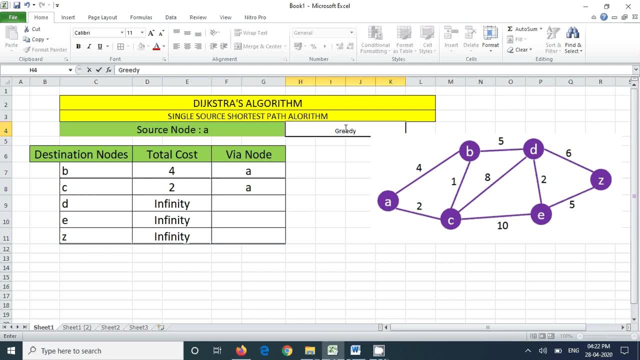 a greedy way of solving. so greedy property is selecting the smallest one. I will just blindly select the smallest one always, but I will yield. this will yield optimal answer. that means correct answer. algorithm correctness will be there just by selecting a smallest every time. so I'll select this one. I will fix. 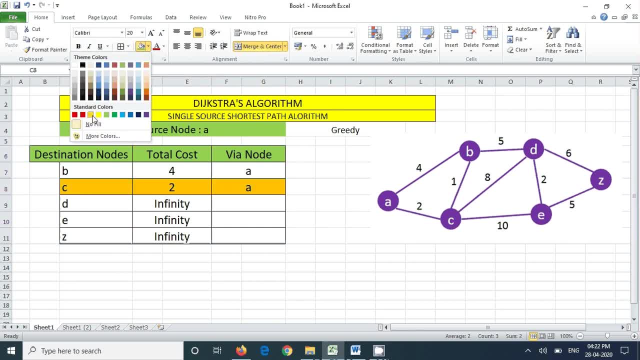 it. this is fix it the fixer. I'll just put the color as say blue for it being fixed it. that means the root to C from a is fixed. C can be reached via a by 2. only. why do they do that? that's what we'll just to do. 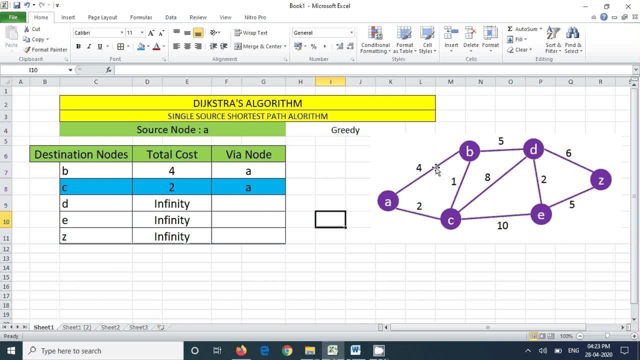 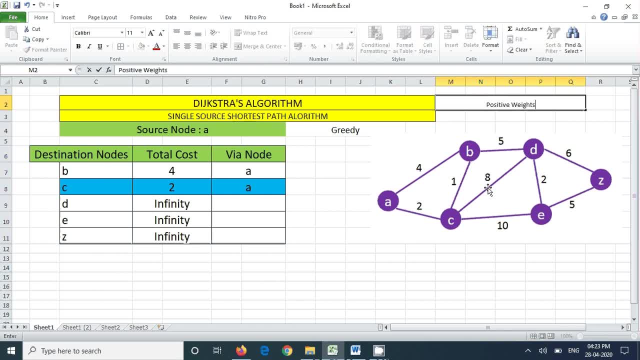 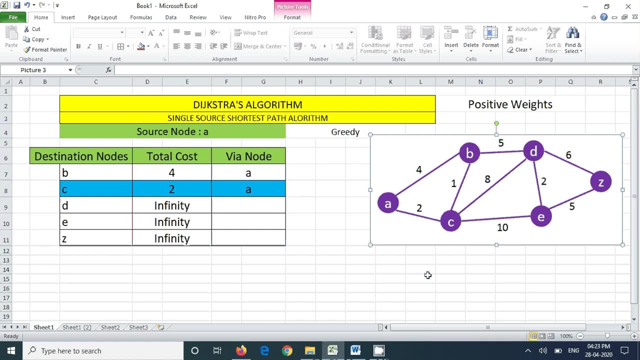 weights, positive weights. it will not work for negative weights, that you remember, Dijkstra's works only for positive weights. let us see why that logic is working, that greedy property without positive weights, how that is working. let us see. so a is going to be with the cost of 4. a is going to C with 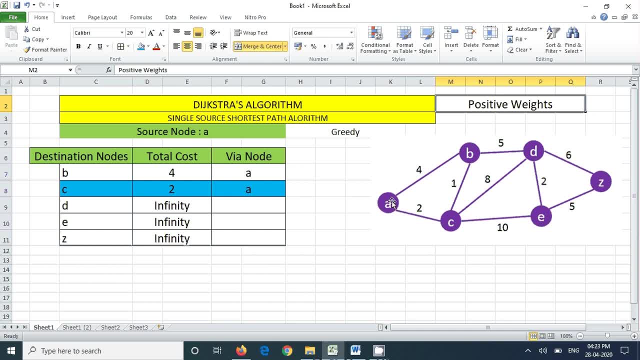 the cost of 2. there are only two outgoing. if I'm reached a, there are only two outgoing edges. I can go by at this edge or I can take this route. if I take this route, it route takes 2 cost. that means I can reach C. 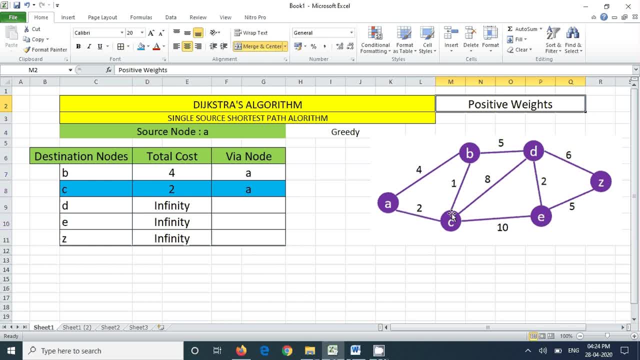 at the cost of 2. these are any other way to read C from a, not following this edge, but less than 2, is it possible? so if I go, why are this way? and if I go to D, then if I come back to C yet to be, then be to D, then D to C if it is less than. 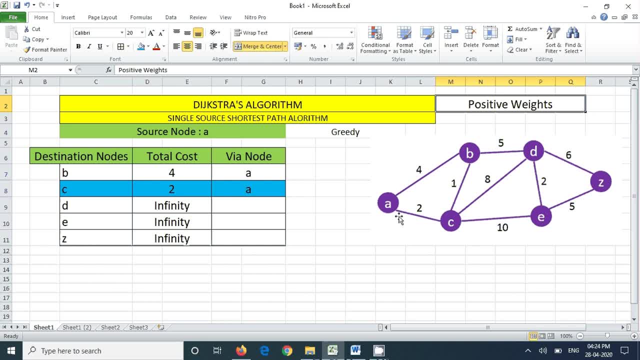 2, then that route should be taken as a path for a, a to c, but it will not work for negative weights. but if there is a negative weight, for example, this is 4, a to b is 4. if this is minus 5, minus 5 plus 4 is minus 1 and this is minus 8, minus. 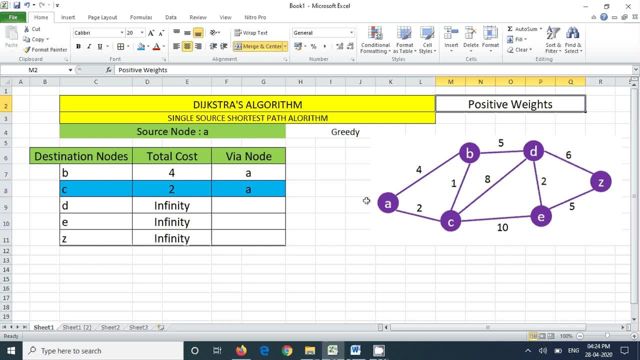 1 plus minus 8 is minus 9, so a to c will be minus 9. here. a to c is 2, so this root i will be taking, but since we are not using my negative weights, dextrose algorithm will always use positive weights. so you cannot come taking this root, which is already more than 2, and come back. 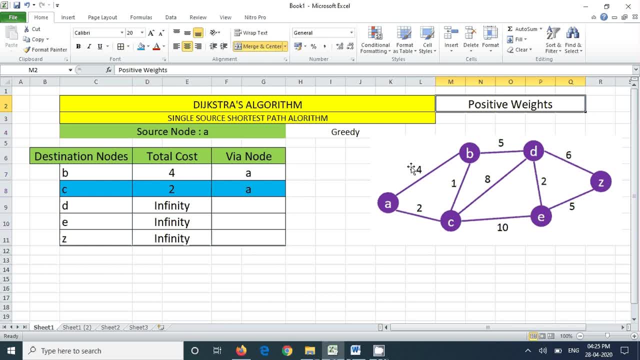 to the c with some other path, which will always be more than at least be equal to 4. so if it is, if it takes already, it's 4, if it takes some other root it will maybe more than 4. so you cannot come to a to c by taking a bigger root, so i have to go to the smaller one only, so smaller one will. 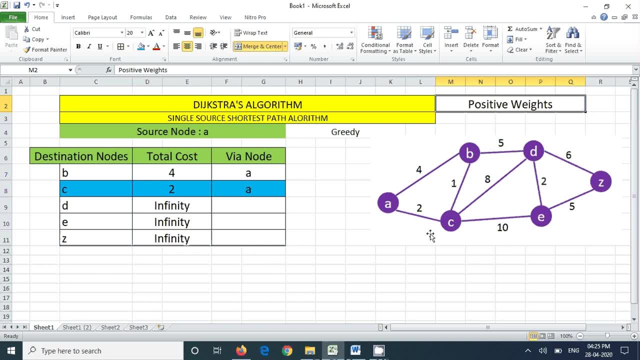 always be correct. so this argument is the base for this dextrose algorithm. so, based on this algorithm, so based on this property of selecting smallest, by this logic, this whole algorithm, the correctness will be maintained. so this is selected as the answer. so c is fixed. a to c is over now, now, once, whatever you have selected recently, whatever that is added to the 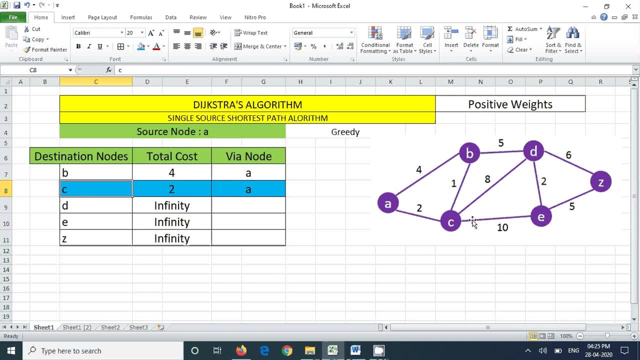 answer set recently. that will be the next scanning point. so i will scan from c. so scan from c. c goes to a. a is the source, so leave it already. we are coming from that way only. so c goes to new nodes we have to discover. c goes to b with the cost of one, so come to c, to come to. 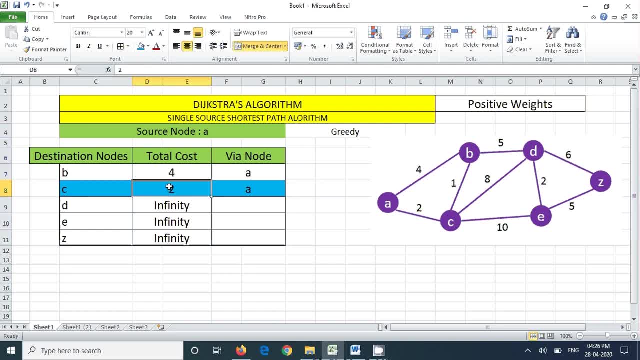 c is what is the cast? because we are doing from a to come to c. cost is total, cost is 2, c is taking one, so 2 plus 1 is 3. because why are we are always starting from a only to come to c? from a is 2, c is: 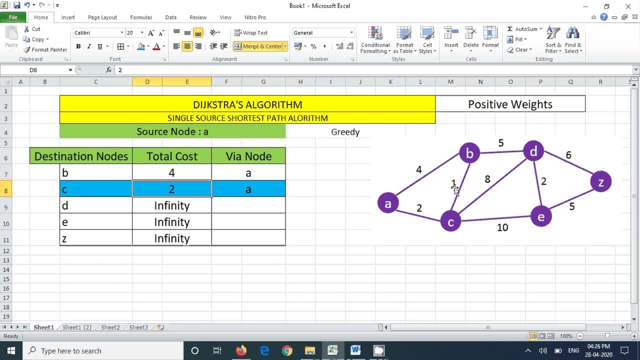 going to be with the cost of 1. so 2 plus 1, 3, 3 is less than 4. that means i have to replace so 3 and But via node is C. The 4 is replaced by 3 and via node is changed. Okay, So this way, Then C can also go to D. D is with the cost of 8.. So to come to C is 2.. To come to C is 2.. Then this is 8.. 8 plus 2, 10.. Totally 10 from A. That is the meaning. 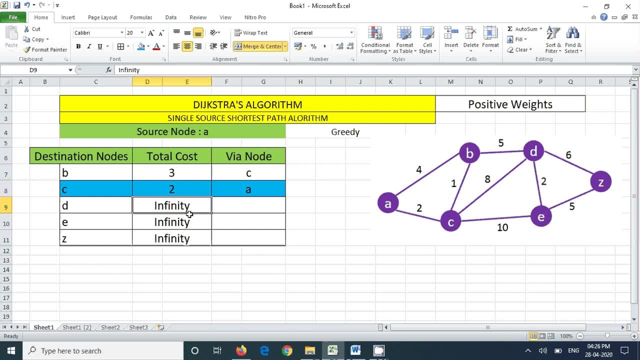 So this is always. the total cost is from A, So 10 is less than infinity. So I am replacing infinity with 10.. So via node is C. for this We are scanning from C. Then C can go to E with the cost of 10.. E, also infinity. So C can go to the cost of 10 to E. So to come to C is 2.. 2 plus 10, 12.. 12 is less than infinity, So I am putting 12.. Via node is C. 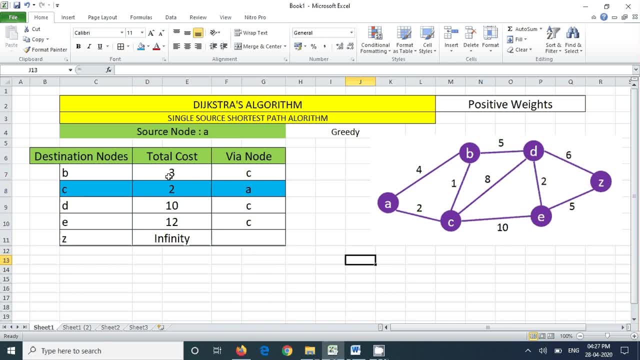 So then that is about it. So this is the possibility: B, D, E. We are all updated. This is replaced. This is replaced the infinity. This is replaced the 4. This is replaced the infinity. So likewise, we have updated the table. Now the same logic goes here also. So we have to select the smallest one and we have to fix it. That is a root from A. So A to B is total 3 via C, A to D is 10.. One more edge: A to E is 12.. 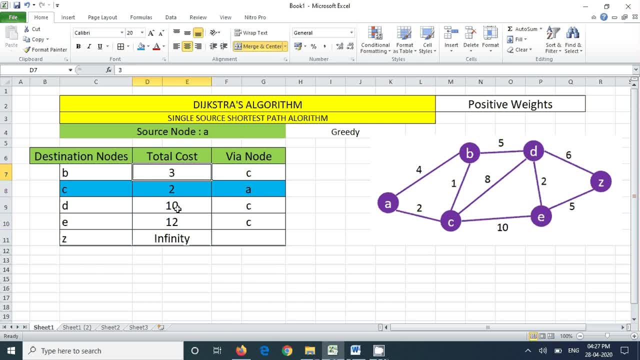 So this is the smallest. So I cannot take D root or E root to come to B lesser than 3.. So we are fixing it. The same property of whatever I explained earlier. The same property. So A to C, A to B is 3.. A to D is 10.. A to E is 12.. So I cannot come to B from A less than 3 by taking D roots. That means it is fixed. So smallest one fixed. 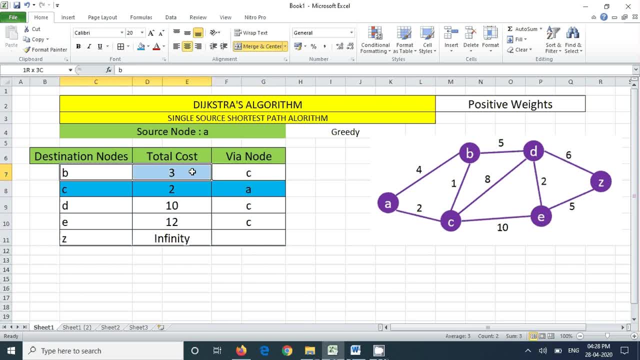 3,, 10,, 12, infinity. Smallest one is 3.. You fix it. I am making it a blue. That means this root is fixed. A to B is found out now. That is the meaning. So recently added is B. now We will scan from B. If you scan from B, B, where it can go? It can go to A, C. A, C are already fixed. This is fixed. A means source fixed. C is already done, So it cannot come via B. That means we are going with a, D, So B is connected to D with the constant. 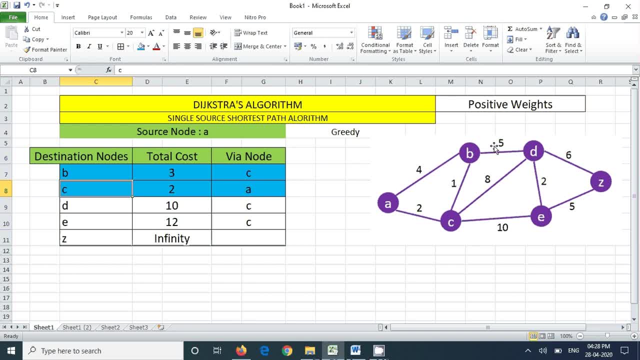 So B is connected to D with the cost of 5.. So B connected to D with the cost of 5.. To come to B is 3.. To come to B from A is 3.. From B to D is 5.. So A to D is 3 plus 5.. 3 plus 5 is 8.. So but already we have a 10 which is more than 8.. That means we have to replace bigger value with 8.. So 8, which is putting 8 via B, Earlier we have put via C. 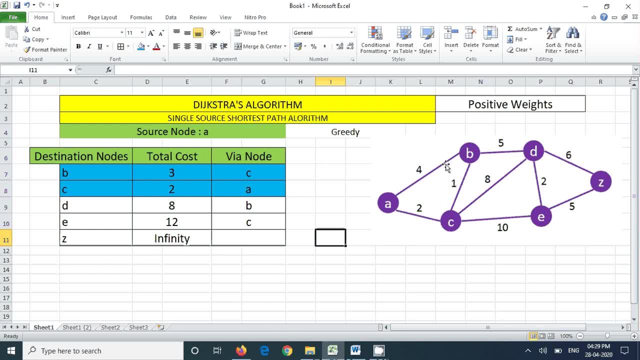 So that is it. That is it. So B cannot go to anywhere else other than A, C and D. A, C. A is a source, C is already in blue, which is fixed. Then D is replaced. D is replaced via B. 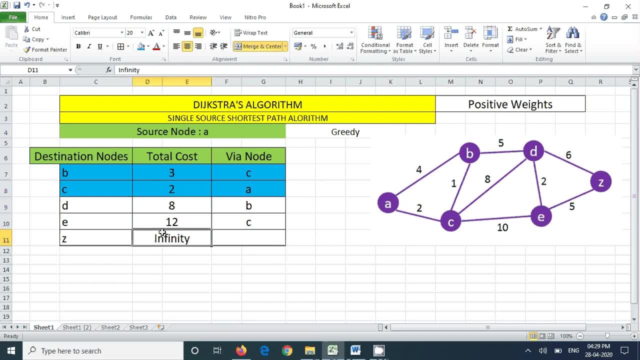 Now next one: Out of these, 8 and 12 and infinity, which is the smallest. So A to D is 8.. A to E is 12.. So I cannot go to A to D by taking 12 roots lesser than 8.. That means this is fixed. 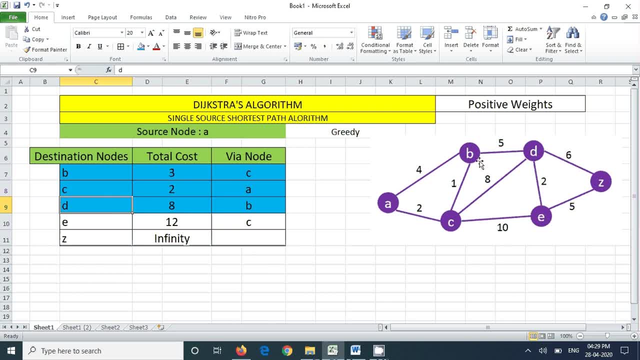 Now D, Now D, Now D. we have to scan from D. D goes to B, B is already added. D goes to C, which is already fixed. Blue, blue. Okay, These 3 are blue fixed. Now D goes to E, with the cost of 2.. To come to D from A, To come to D from A, is 8.. Then from D to E is 2.. So 8 plus 2 is 10.. So 10 to E via D, So it is less than 12.. So I am replacing 12 with 10 via D. 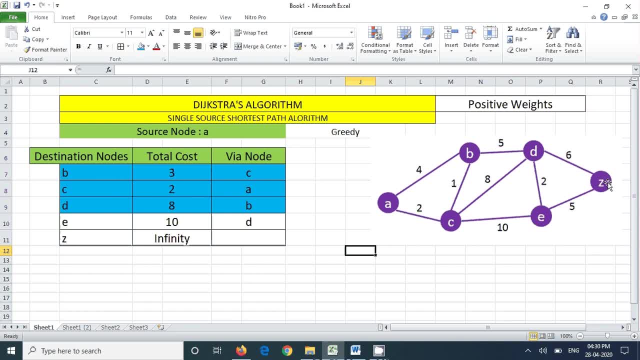 And D goes to Z. This is the first time we are encountering Z destination. D goes to C, Z with the cost of 6.. So to come to D is 8.. 8 plus 6 is 14.. So 14 is less than infinity. So I am replacing infinity with 14. and via node is D. 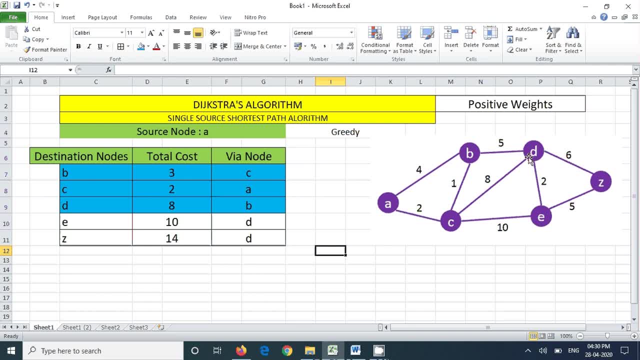 D can go to E with the cost of 12.. This is already done. This is already done And Z is Done now Newly added. Okay, Now we have left out with 2 things: 10 and 14.. A to E is 10.. A to Z is 14.. So I cannot go to E from A less than 10 by taking Z root. That means this: you have to take it as a blue one. 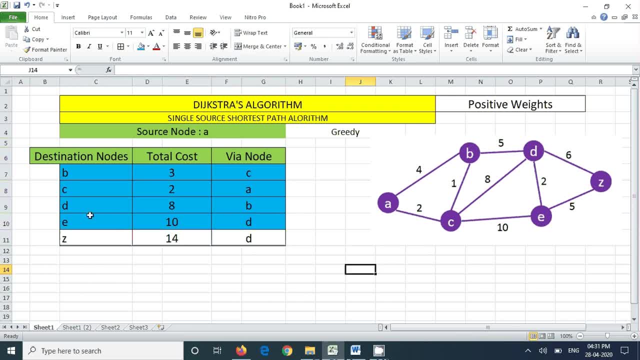 Let us take it into answer. set E is fixed, A to E is fixed with 10.. Now recently added is E. So we are scanning from E. So E to Z is 5. To E To E is 10.. A to E is 10.. E to Z is 5.. So A to Z is 15.. But 15 is more than 14.. So you should not replace this value. So E goes to Z. That is only to replace E to D. Already D is fixed. That based on the property E to C already fixed. 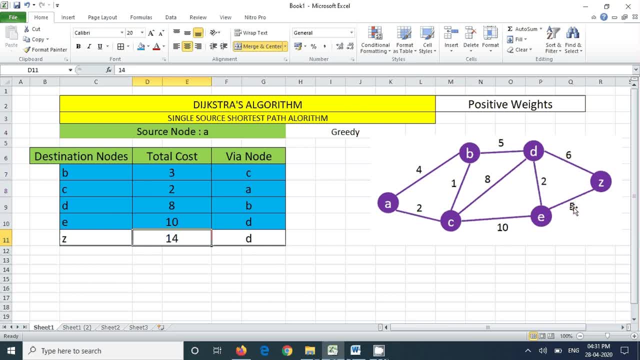 So only thing is it can go to Z with the cost of 15. So to come to, E is 10.. Then 5, 15. But 15 is more than 14. So via D is the best rule. So that is also fixed. That is done. 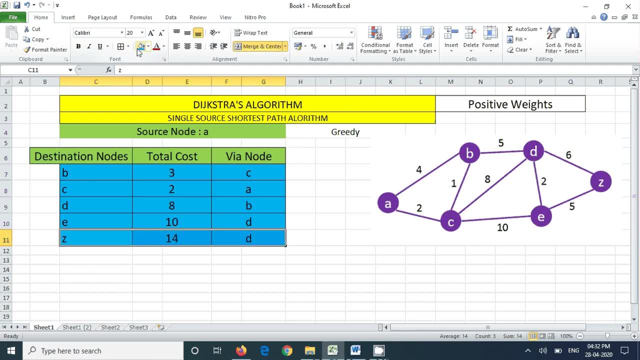 Now, which is the only one left out. This is the only one left out. We are added to the answer. set A to Z is 14 via. So this table is now formed From this one. we are going to find the path. What is the path? 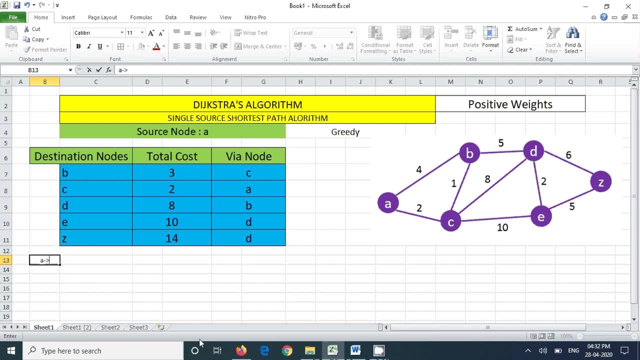 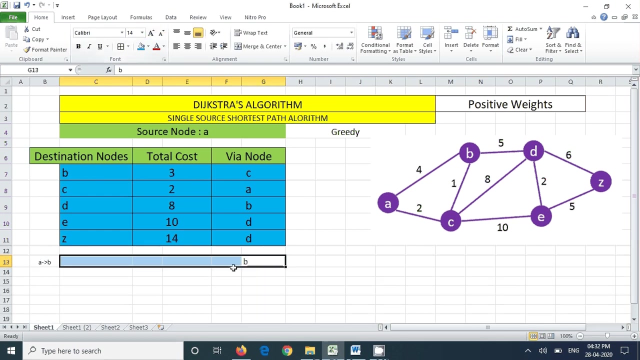 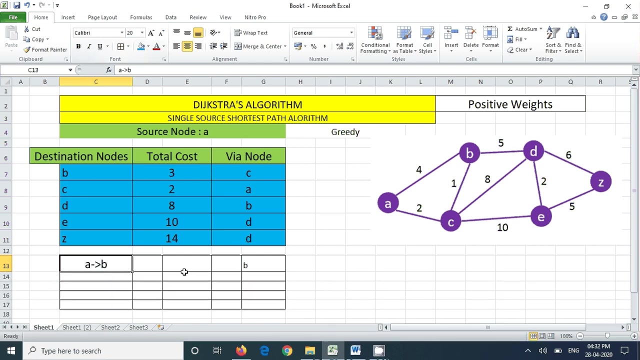 A to Z. A is the source, node A to B. You just see what is the path for A to B. You can reach B. Destination is B. Destination is B, Node B. We will find the paths A to B. What is the path for A to B. So reach is B. B can be reached via. It is known: Total cost is 3.. Total cost is 3.. B can be reached via C. So first to go to C Via C. 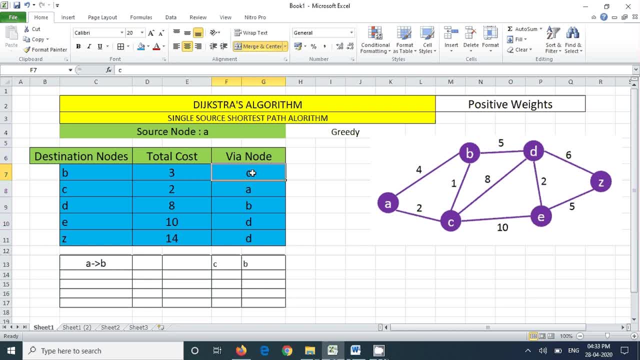 So B can be reached via C, That means then you have to C Go to this one C, The road C Node can be reached via A. So that means you have to put like this: So this is the path. 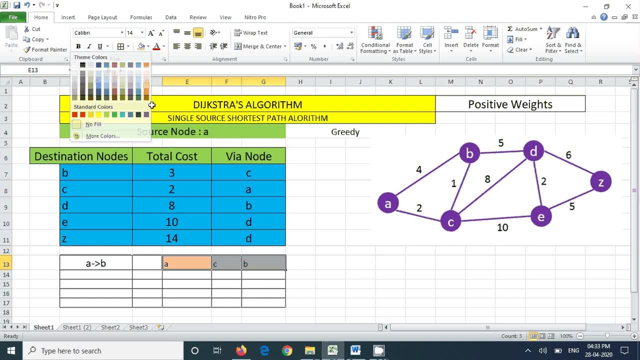 A Path A to B is A to B positive, A to C, Then C to B, A to C, Then C to B. That is the path. So how to start. I will tell again How to do. 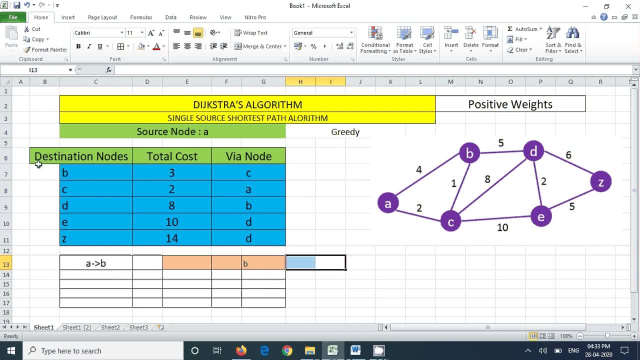 Just, you have to find via B, So destination. you put it here. You see the table. The table: What is the via node for to reach B? The previous node is C. But how will you reach C? Via is A. A is the source node. So you are stopping, You are not going further. A is the source node Till you reach the source node. you have to follow this approach. Now, A to C, A to C, What is the route? Let us see. So C is the destination, C is the destination. 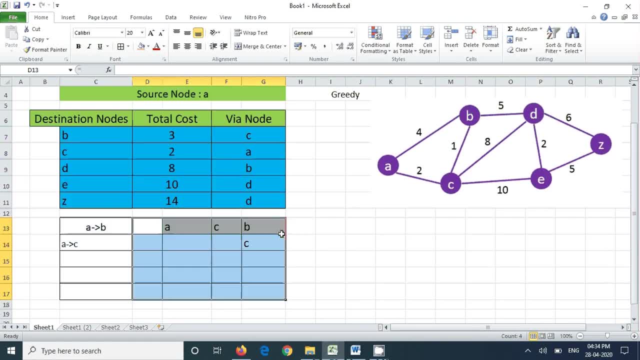 C is the destination. A to C. To come to C, it is A, So directly you just put it, No problem, We reach the source node. So that means we fix it. So A to C is just route. Path is A, C, A, B. path is A, C, B, A, C B. These are vertices, Vertices, path. 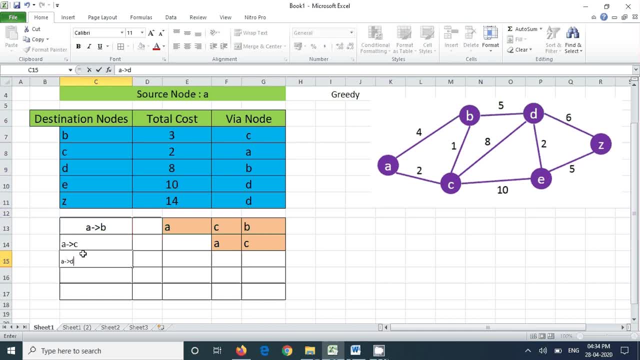 Then A to D. We will just see how A to D is. A to D, D is the destination. You put it here. You see the table: D can be reached via B. So put the via B here, Go to B. B can be reached via C. Put a C here, Go to C. C can be reached via A, But the total cost is This: total cost A to B. total cost is 3.. That is A to C. total cost is 2.. 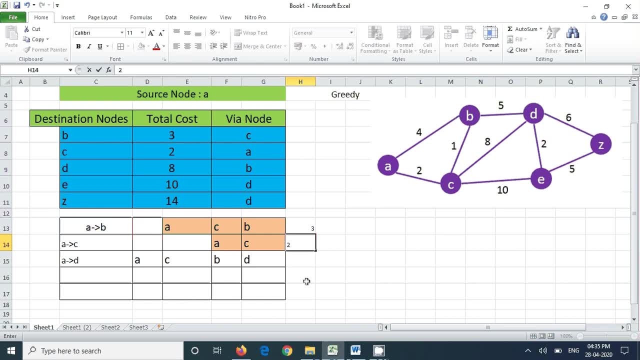 2. A to D. total cost is 8.. Okay, That you can find out easily. You see, this one. This is the route for A to D. A to D. D is here. How will you go A to C First? you go to A to C with the cost of 2.. 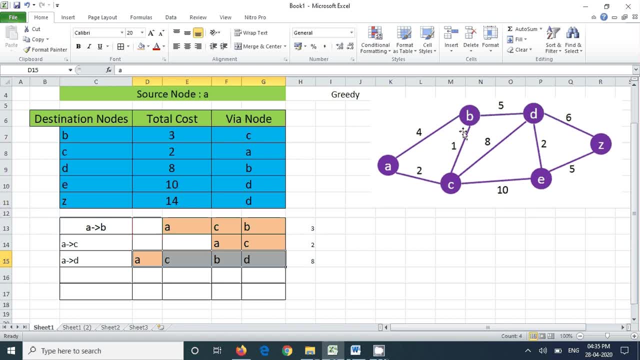 Then C to B with the cost of 1.. 3. Then B to D with the cost of 5.. So A to B, 2 plus 1 plus 5.. Totally 8.. This is A to C. A to C is 2 directly. 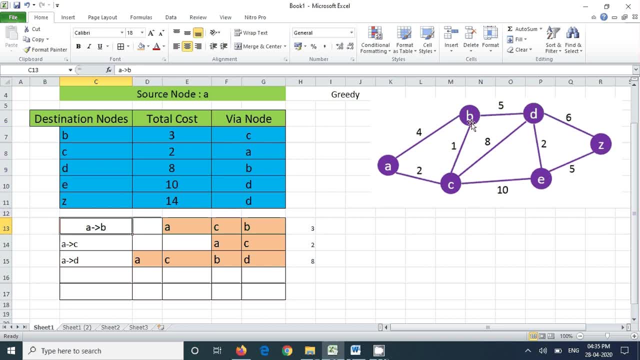 A to B is A, C and C- B. A, C is 2.. C, B is 1.. 3. Total cost is 3.. So this gives the total cost. That is what I put total cost here. A to E. Now you just see for A to E. 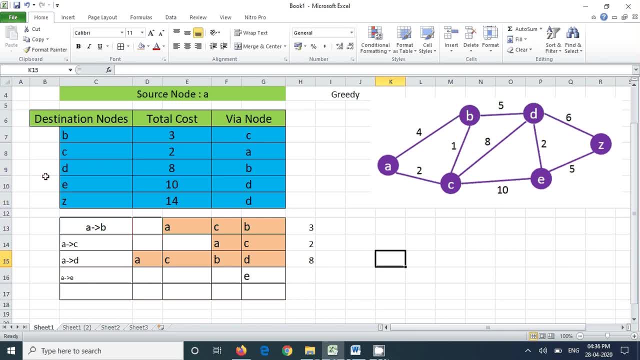 What is the cost for A to E? You put the E here, Destination E can be reached via D. You put D here. D can be reached via B. Put the B here. B can be reached via C. Then C can be reached via A. 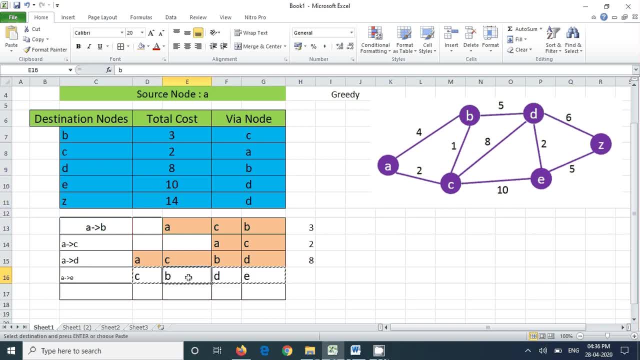 I will just A. This is the roots, This is the root for. So I will tell again. So here I will put the destination: Destination is E. Destination is E, A to E. we have to find it. What is the path? 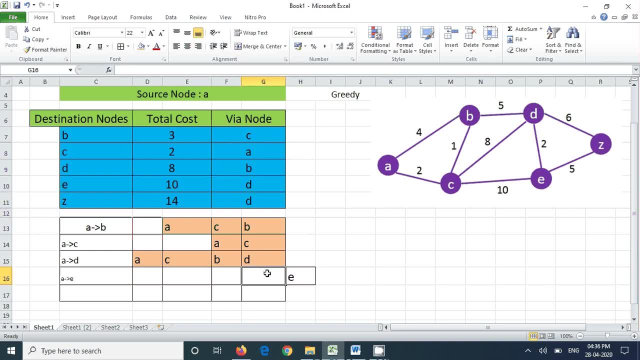 You see the table E can be reached via D. So previous node is D. So how the D is reached. D's previous node is B. You put the B here. What is the previous node of B? B's previous node is C. 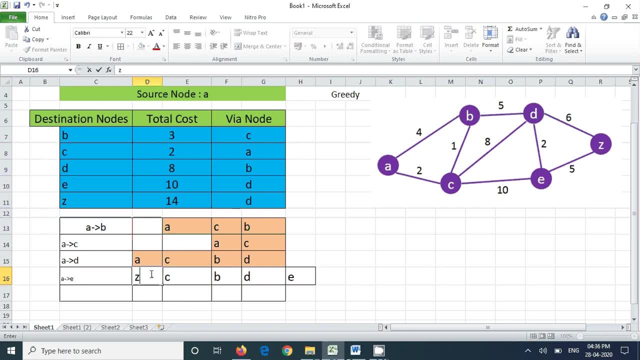 What is the previous node of C? C's previous node is A. So this is the path. The path is A to E, is A to C, AC Then CB Edge, AC edge, Then CB edge, Then BD edge. 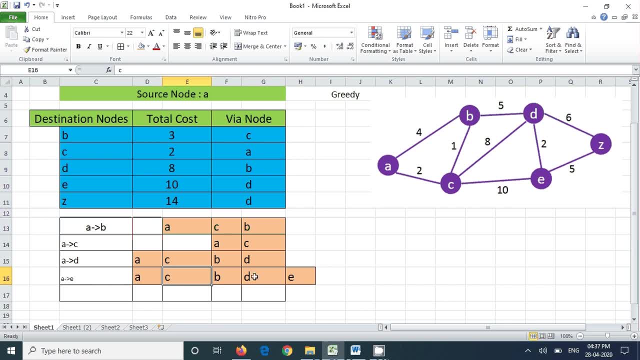 Then DE edge, So 4 edges: 1,, 2,, 3, 4.. You have to cross 4 edges to reach E, So A to C, A to C. You have to go like this, Then CB. 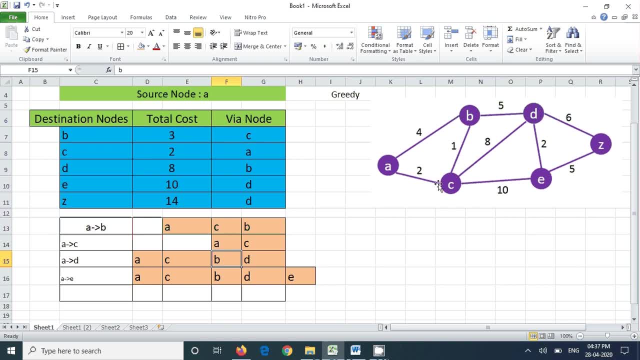 Then BD, Then DE. That means 2 plus 1, 3.. 3 plus 5, 8.. 8 plus 2, 10. Totally 10.. 10 is the cost here. So that's A to E's. 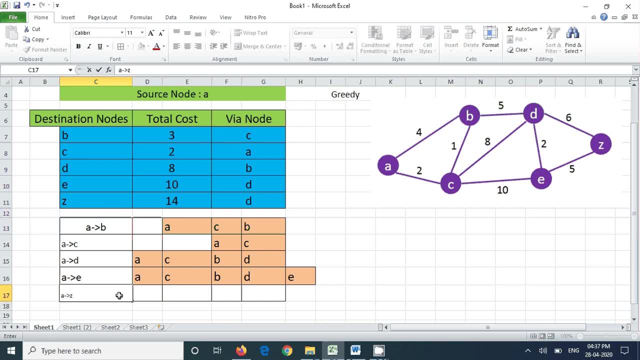 Now the same way A to Z. What is the cost of reaching Z from A And what's the Total cost is 14.. That is found out, But what's the path? You have to just see: Reaching Z. 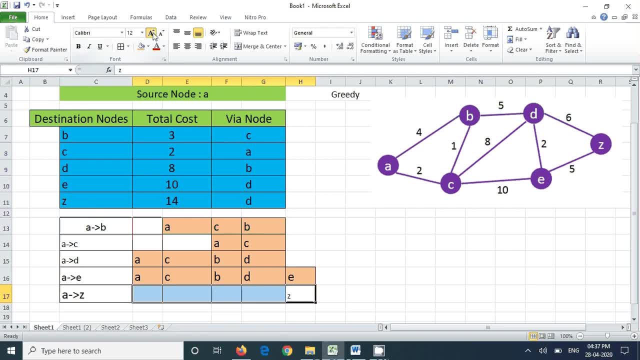 OK, Reaching is Z. How you are reaching Z. Let us see: Destination is Z. Go to Z. Z can be reached via D. D can be reached via B. B can be reached via C. Put C. C can be reached via A. 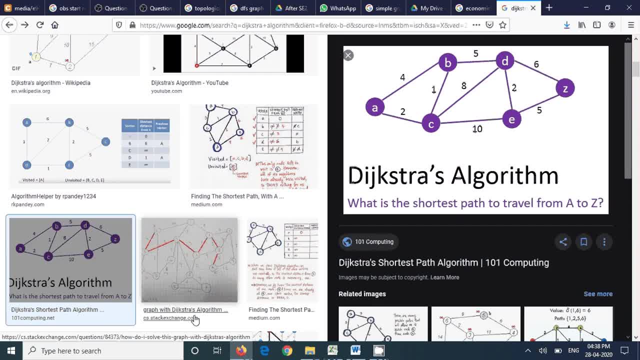 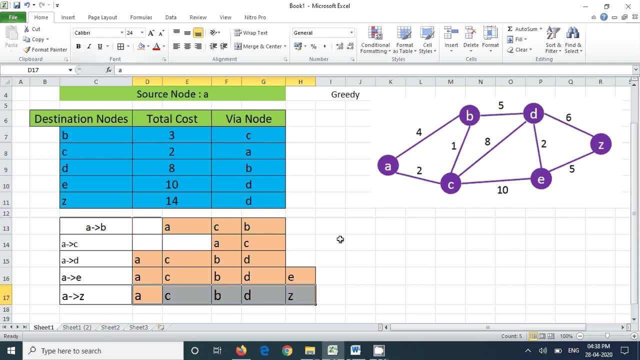 So when you reach A, you have to stop Because that's a, That's a source node. okay, so this is the path. these are all the path. path is acb. path is ac, acbd. likewise, we are putting the path. so from this table you have to extract the path. the table gives the total cost from a to. 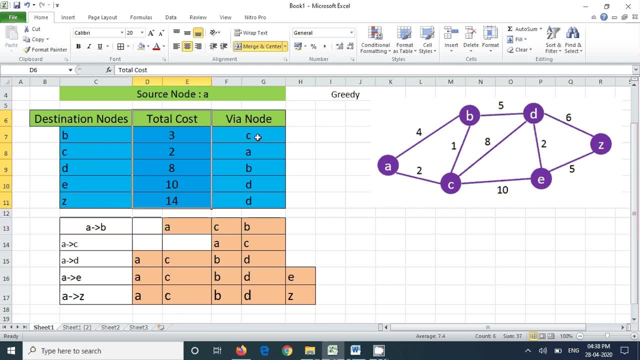 b, a to c, the total cost is given and the yr node is given. yr node means just a previous node. you cannot get the full path. so full path derivation: you have to just write a simple logic to get the derivation of full path a. b path is a to c, then cb, it's edge to edge.